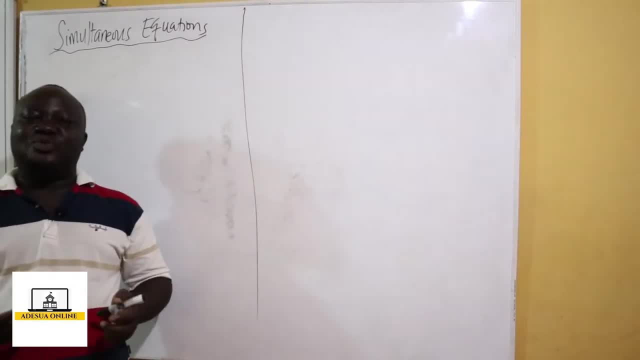 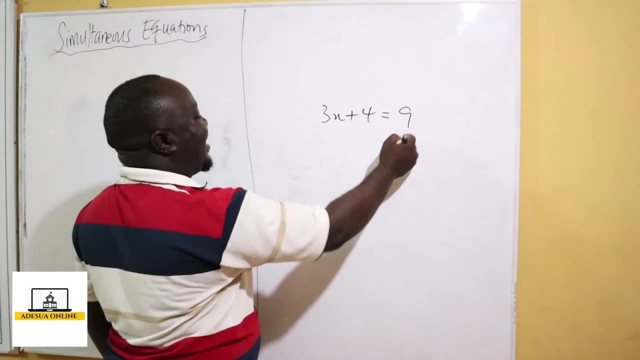 about simultaneous equation. we are talking about having two variables, x and y. Earlier on we learned that if we have 3x plus 4 is equal to, let's say, 9, and we have been asked to solve for x. we say 3x. 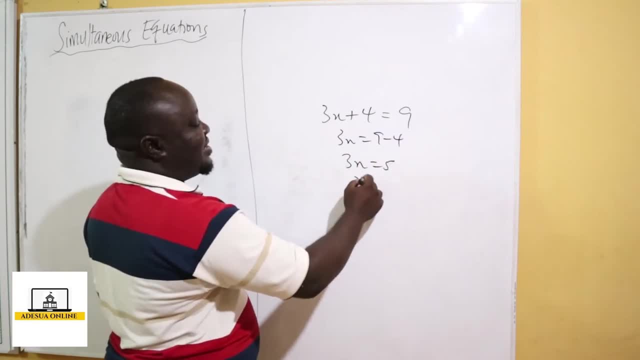 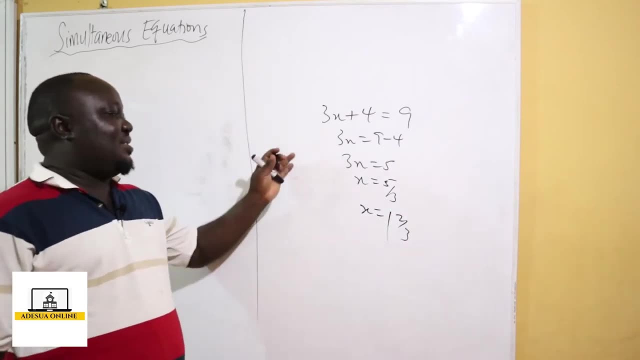 is equal to 9 minus 4, 3x is equal to 5, x is equal to 5 over 3, or x is equal to, let's say, 1 over 2 over 3.. Now, this is an equation given to you which has only one variable, and you have been asked to. 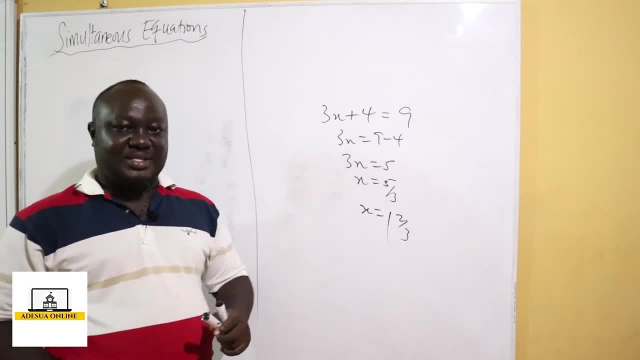 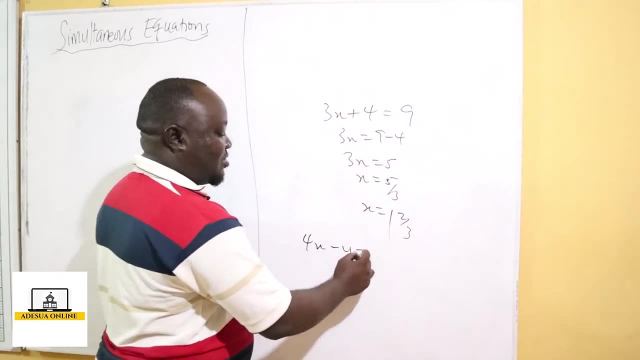 find the solution to that one variable, which is the variable x. Now, in a situation where you are given two variables, x and y, you can be given, let's say, 4x minus y is equal to 6, then x plus 3y. 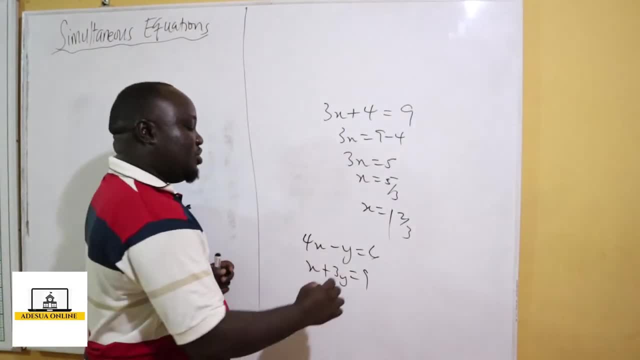 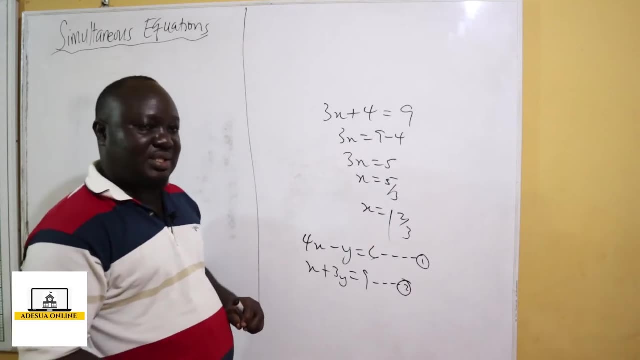 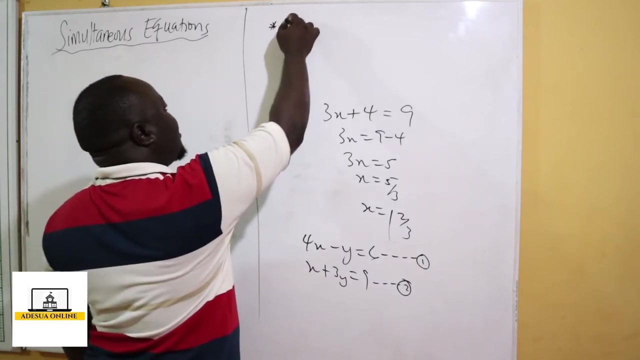 is equal to 9.. You are supposed to solve for x and y, So we identify this as equation 1 and this is equation 2.. What happens in this situation is we have three different methods of solving simultaneous equation. We have what we call the graphical method. We also have what we call the 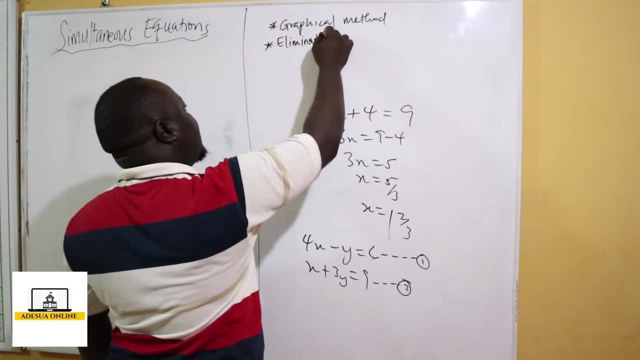 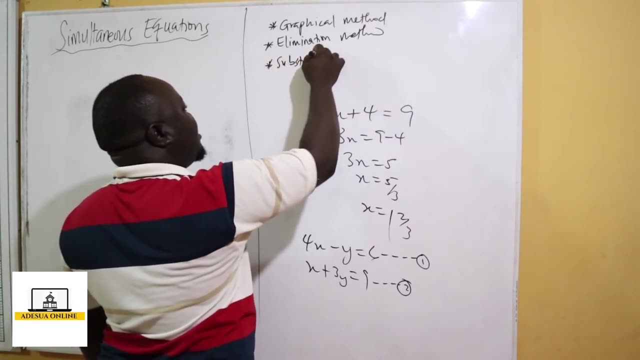 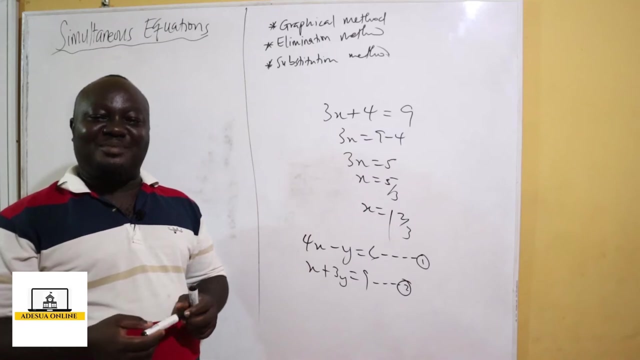 elimination method, And then we have the substitution method. So we are going to have a look at all these three methods of solving simultaneous equation. So let's start with the graphical method Now. for example, if we have, using a scale of 2 centimeters, 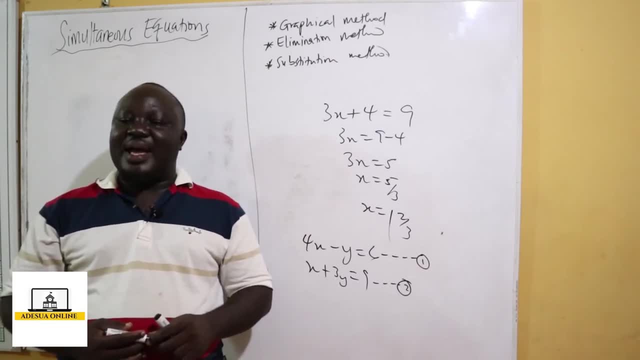 to 1 unit on the x-axis and 2 centimeters to 2 units on the y-axis. draw the graph for the straight lines: y plus 2x is equal to 1 and y minus 3x is equal to 1.. So we have a scale of 2 centimeters. 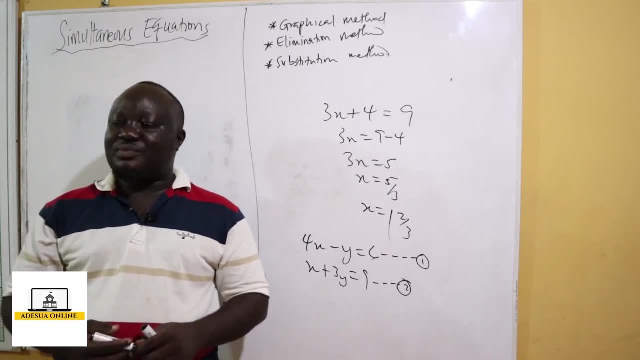 to 1 on the y-axis and 2 on the y-axis, And then we start from the last two points on the y-axis. So what we have to do is we have to find the coordinates of the point of intersection, So we move to our graph board and then we solve this simultaneously. Now, before we solve this, what we 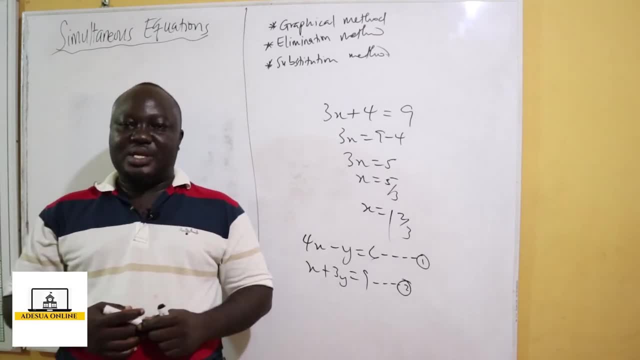 need to do is we need to find values of x and y which should correspond to our table, and then we plot it And then, when we find the points of intersection, then we write them down and that will be our solution. Sometimes, when you have an equation, sometimes it's all you can find: the x and y intercepts. 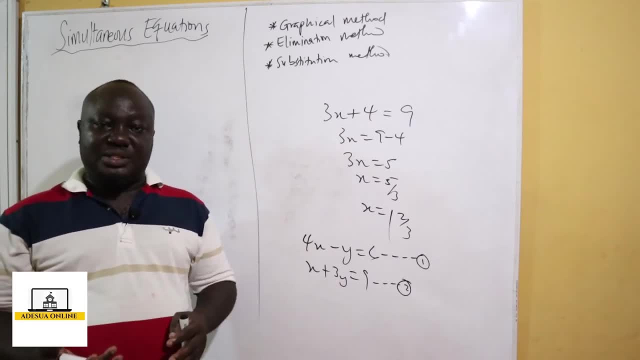 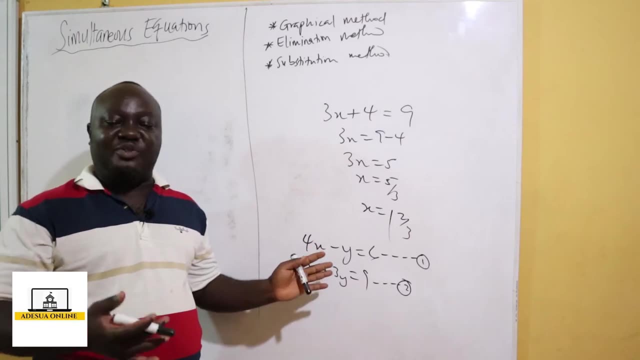 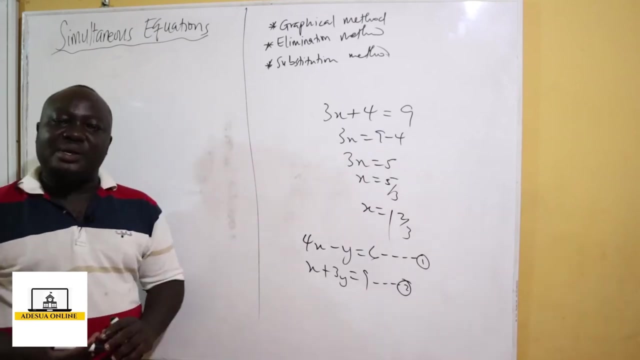 But in this case I would advise you only pick 3 points or 2 points on the Oxy plane and then you just add it, plot it as your x values, and then you find the corresponding y values and then you plot it. Now one thing is for any straight line, any 2 points you pick, the gradient is always. 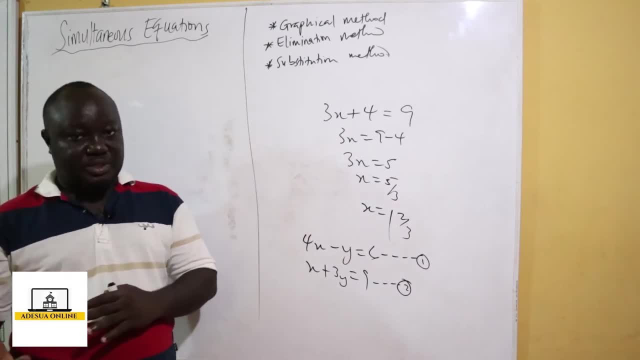 what The same. So you choose to get 2 points or 3 points or, if you like, 4 points. So it depends on you what you want. So I'm going to pick 3 points on the Oxy plane and I'm going to find the values of what. 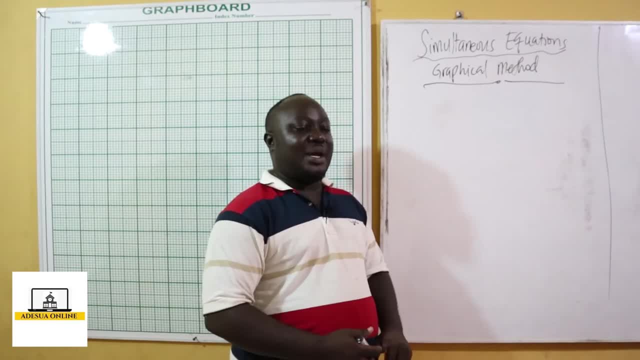 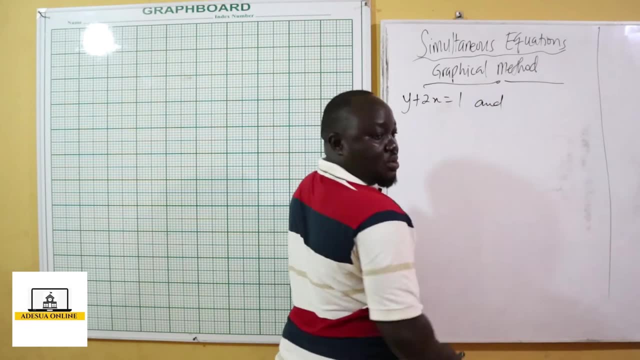 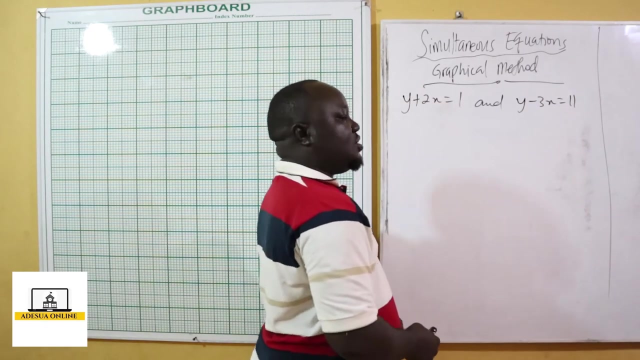 x and y. So we are going to solve, for y plus 2x is equal to 1, as our first equation, and y minus 3x is equal to 11,. y minus 3x is equal to 11 as our second equation. 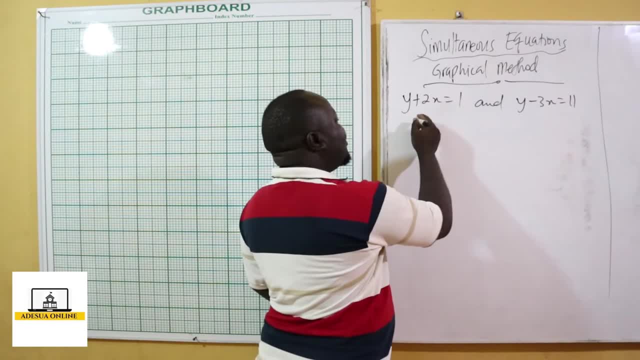 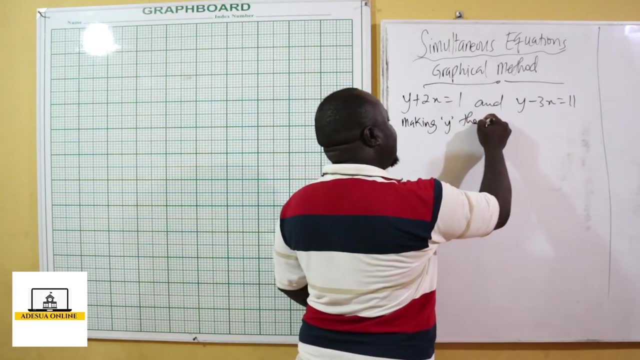 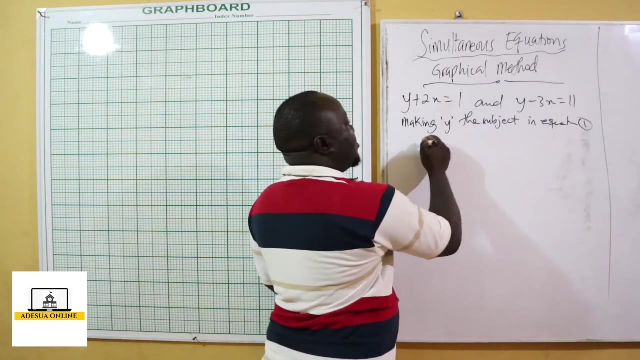 So what we are going to do is We are going to make y the subject, So making y the subject from equation 1.. So making y the subject, Making y the subject in equation 1.. We shall have, This is our equation 1 and then this is our equation 2.. 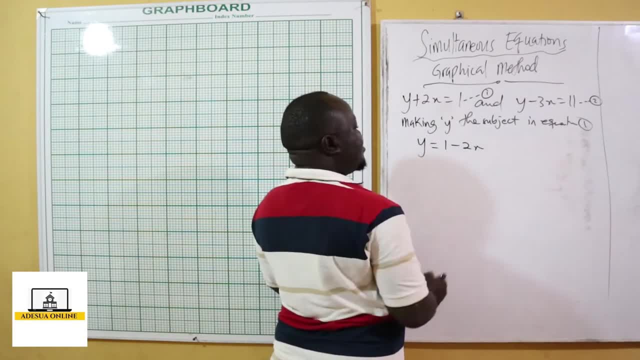 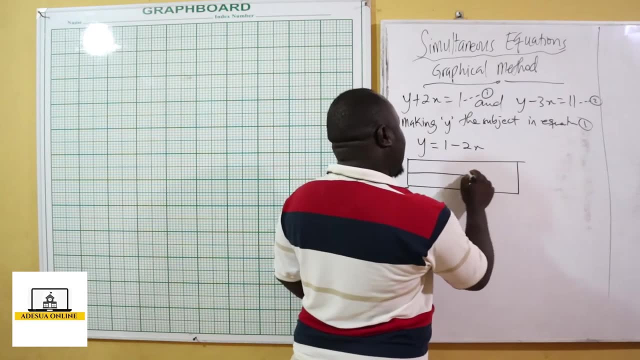 We shall have. y is equal to 1 minus 2x. Now I'm going to pick 3 values of x and 3 values of y. I'm going to put them on the Oxy plane and then put them here. I have x and y. 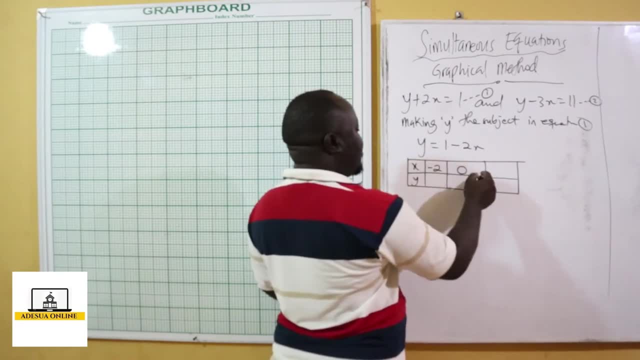 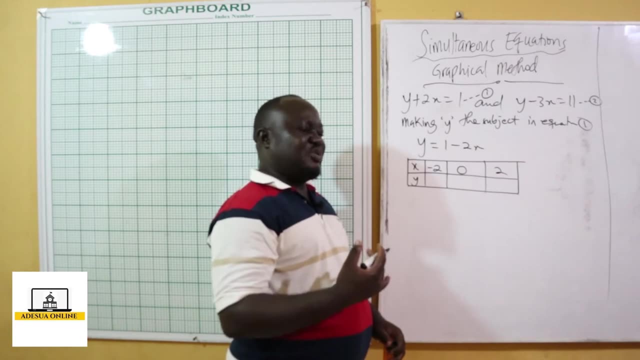 So let's assume I have negative 2,, 0 and 2.. Okay, I have the x values of negative 2,, 0 and 2.. So don't let your x values move so far away. Let it just be around. 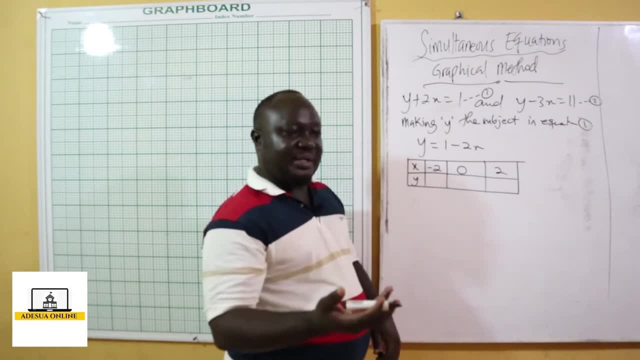 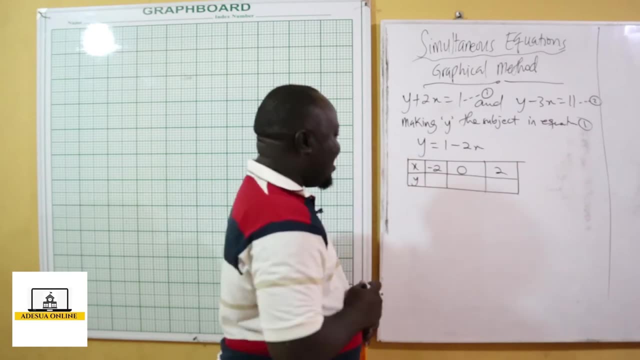 You can pick negative 4,, 0 and 3.. Anything you want to pick, just pick them. But just be, you know a little matured about it, You understand. So picking negative 2,, 0 and 2.. 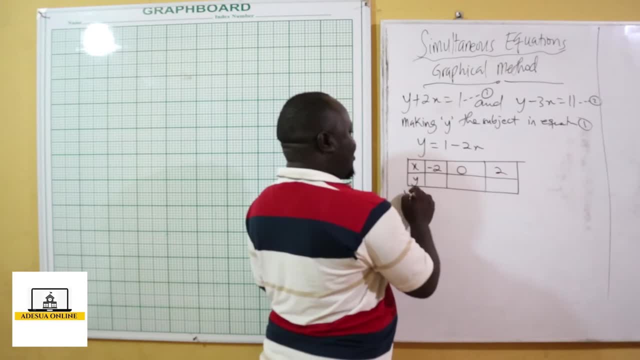 When x is negative 2,. I put it into this equation: If I have y equals to 1 minus 2x, When x is equal to negative 2, my y will be equal to 1 minus 2 times negative 2, which. 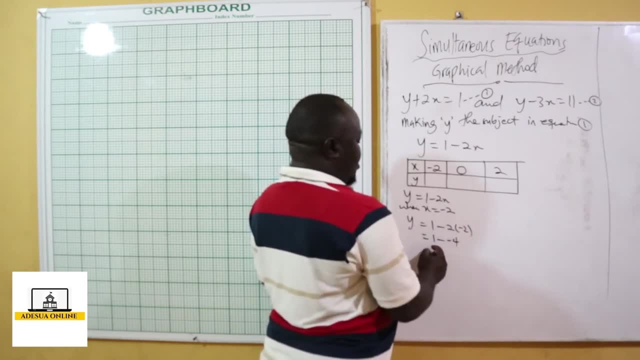 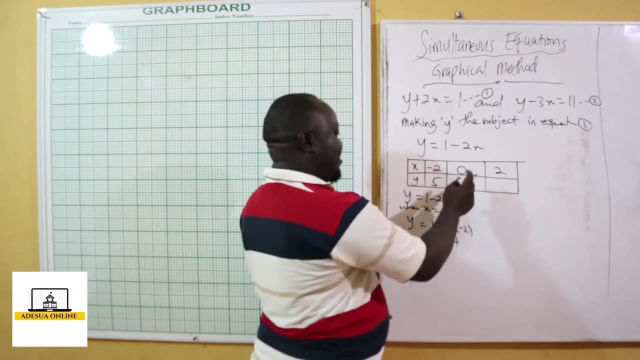 will be 1 minus 2 times negative. 2 is negative 4, which will give me positive 5.. So, when x is negative, 2, y is 5.. The same way when x is 0.. Okay, When x is 0, 2 times 0 is 0. 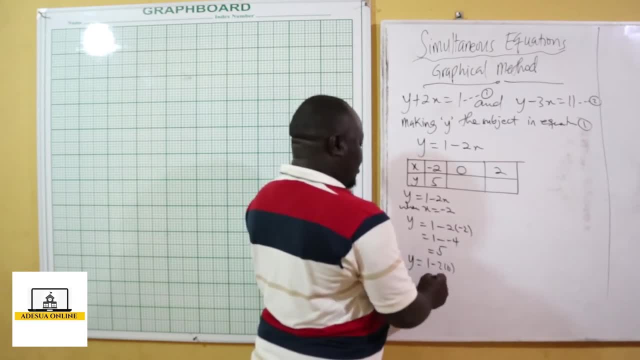 y will be equal to 1.. So I have: y equals to 1 minus 2 times 0. So y will be equal to 1.. Well, when x is 0, y is 1.. And then we go for the last one. 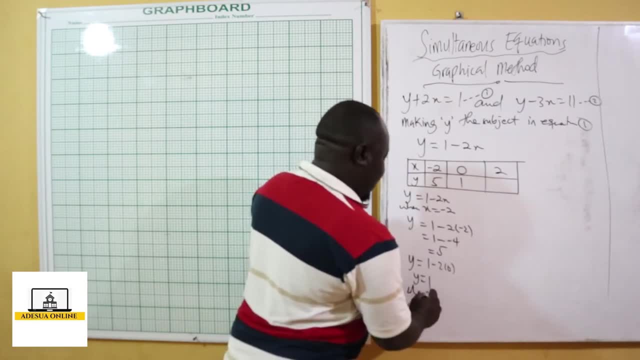 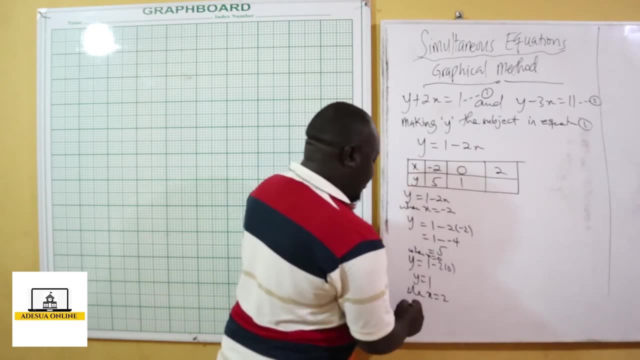 When x is equal to positive 2.. So when x is equal to 2.. This is when x is equal to 0. So when x is equal to 2, we put it back into the equation: y is equal to 1 minus 2 times 2.. 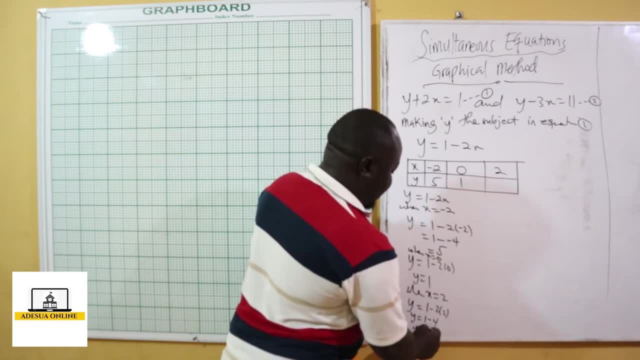 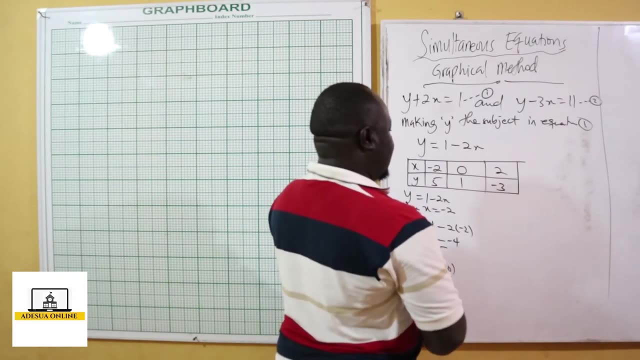 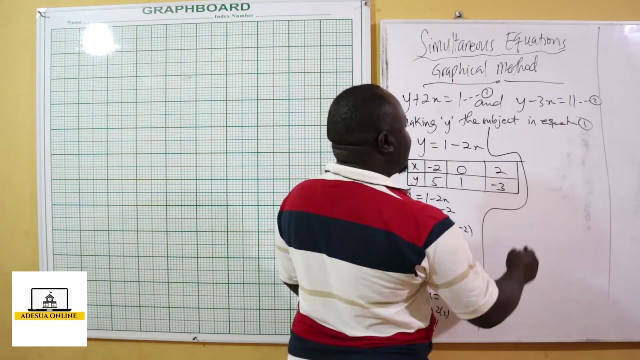 y will be equal to 1 minus 4.. y will be equal to 2.. y is equal to minus 3.. So when x is 2, y is minus 3.. So that is for our first equation. Then we move to the second equation, which is y minus 3x is equal to 11.. 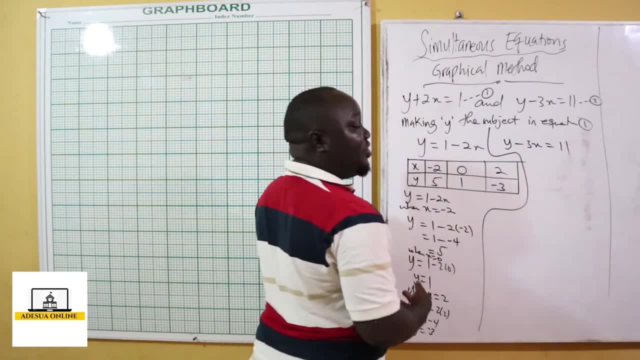 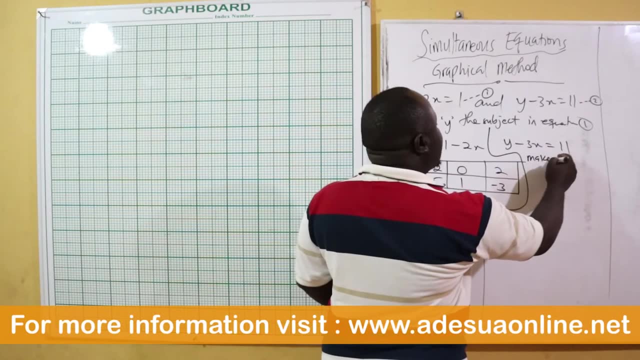 So y minus 3x is equal to 11.. The same thing: We are going to make x the subject of this relation. So making x the subject. So make Sorry, Making y the subject. Make y the subject. Okay. 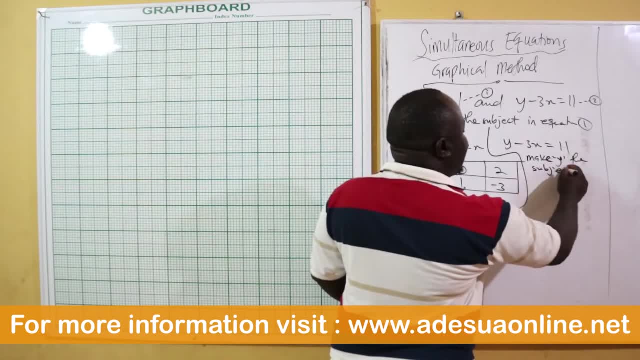 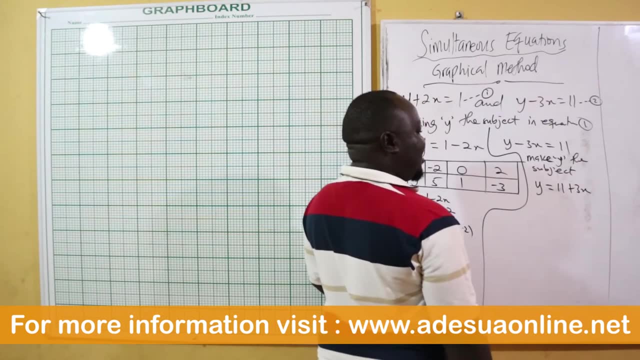 Make y the subject, Make y the subject. We shall have y to be equal to 11 plus 3x. So if y is equal to 11 plus 3x, we are going to pick three values of x and then three values. 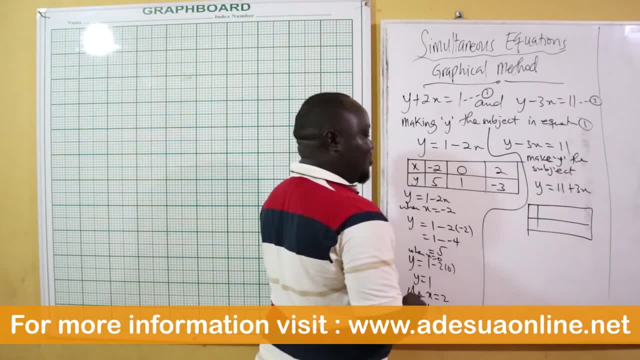 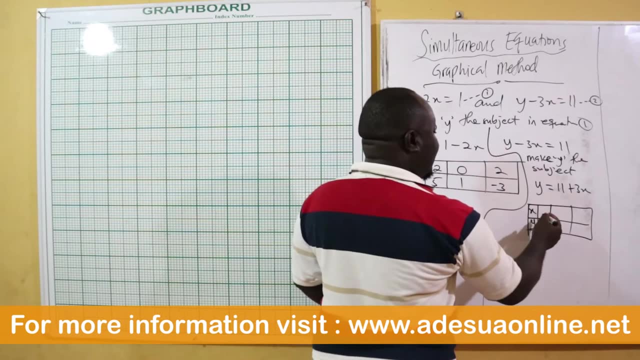 of what Values corresponding, we find the corresponding values of y. So if I have my x and my y, let's say I pick negative 1 or negative 2.. Negative 2. 0.. x, 0.. And then let's say 3.. 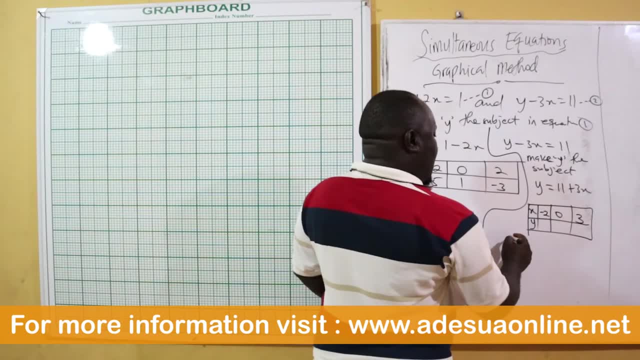 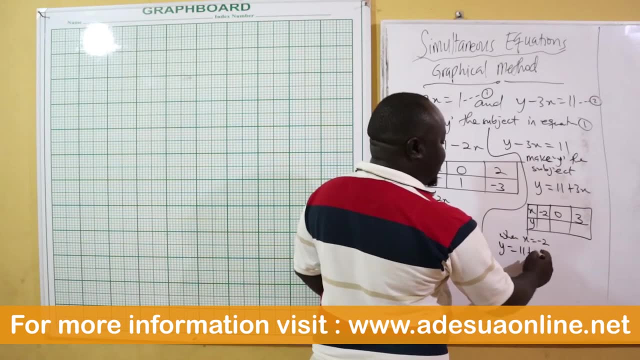 Negative 2, 0 and 3.. So let's go. y will be equal to. When x is equal to negative 2, I will have y to be equal to 11 plus 3 times negative 2.. y will be equal to 11 minus 6.. 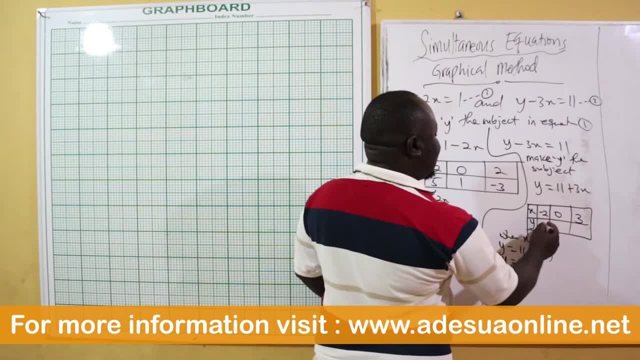 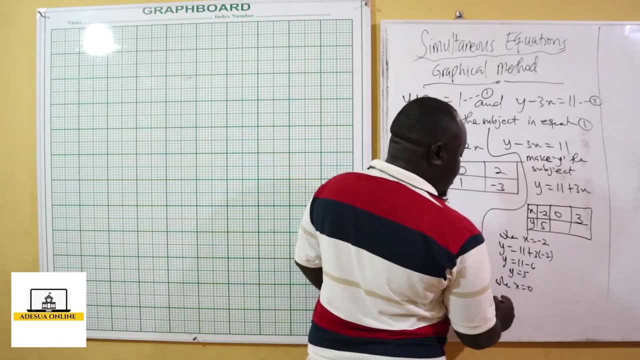 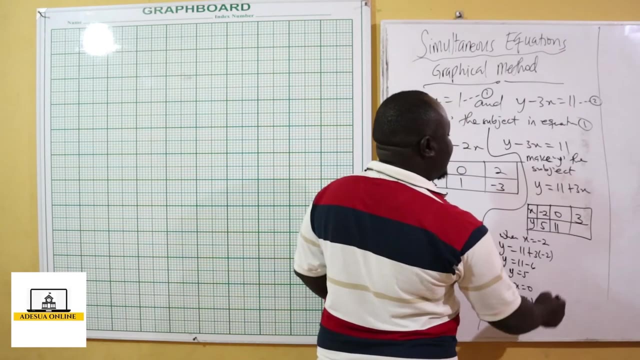 y is equal to what 11 minus 6 is 5.. So when x is negative, 2, y is 5.. And then when x is 0. When x is equal to 0. y will be equal to to 11 plus 3 times 0,. y will be equal to what 11.. So when x is 0, y is 11.. And then the 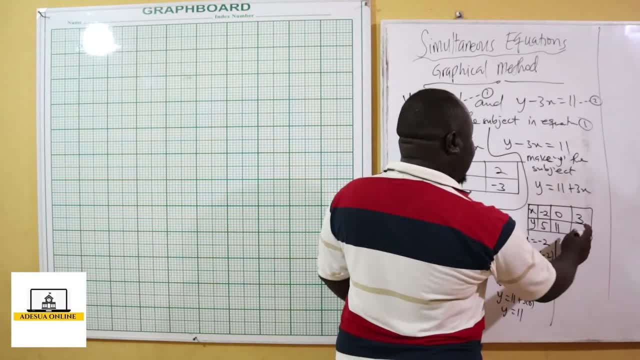 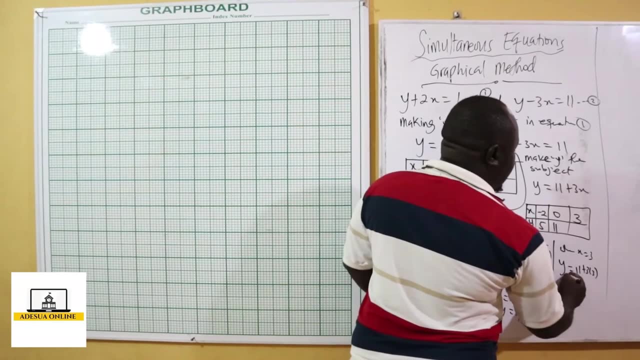 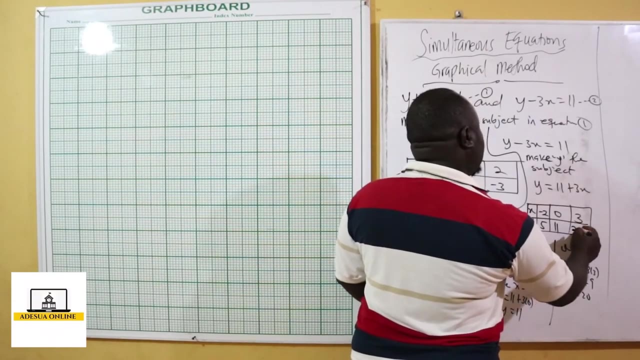 last one: when x is equal to 3, y will be equal to 11 plus 3 times 3, y will be equal to 11 plus 3, 3, 9, y will be equal to 20.. So, when x is 3, y is 20.. Now, with these corresponding 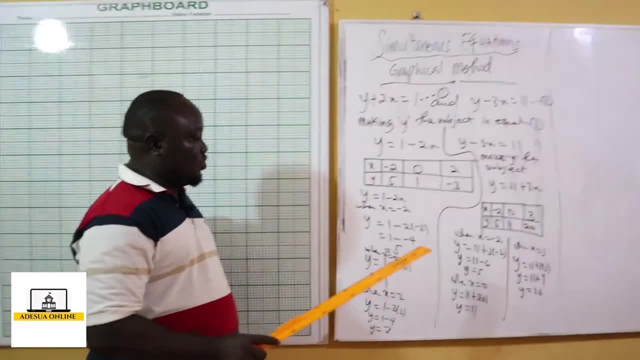 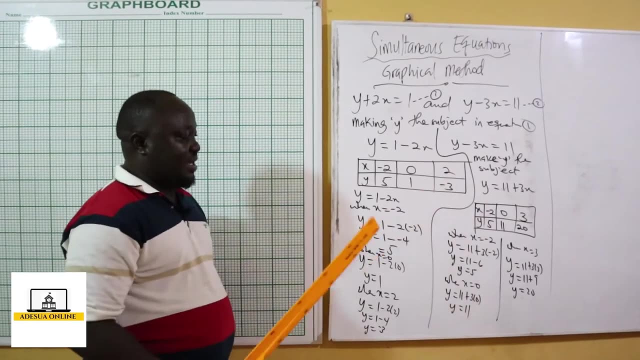 values of x and y. you know: when x is negative, 2, y is 5.. When x is 0, y is 1.. When x is 2, y is negative, 3.. When you catch the second equation: when x is negative, 2, y is 5.. When 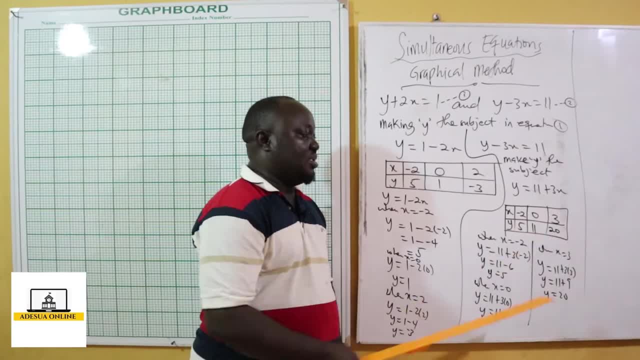 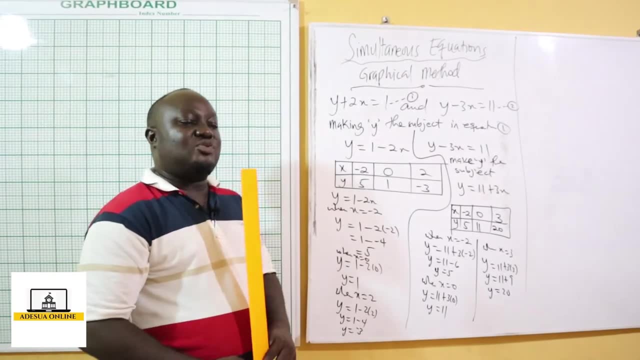 x is 0,, y is 11.. And when x is 3,, y is 20.. We are going to plot this point on our Oxy plane And from the question we are told that we should have 2 centimeters to 1 unit. 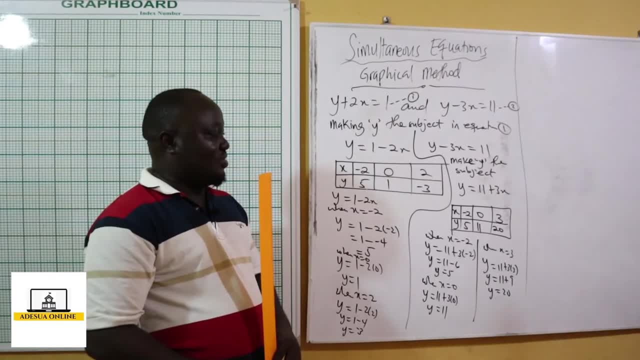 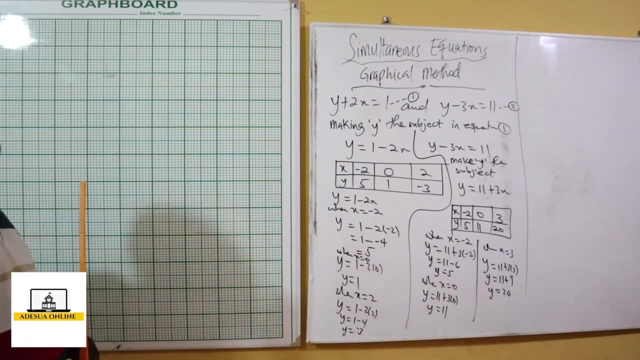 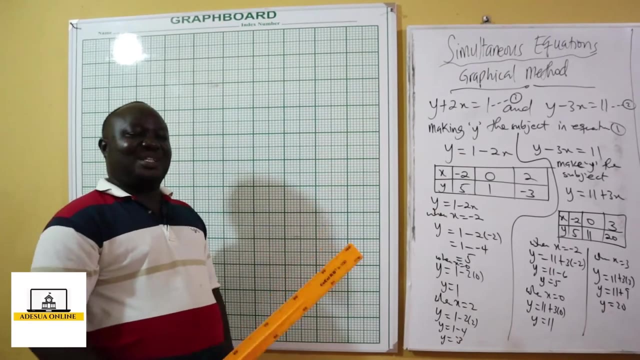 on the x-axis and 2 centimeters on the y-axis. So we are going to plot this point on our Oxy plane. So we have 2 centimeters to 2 units on the y-axis, So let's find the corresponding values of x and y. So because we have 2 centimeters to 1 unit on the x-axis, my values of x range. 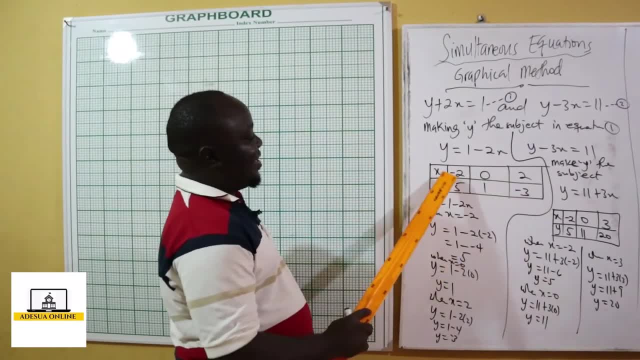 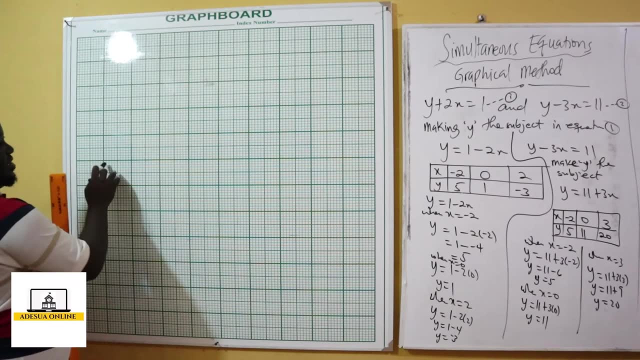 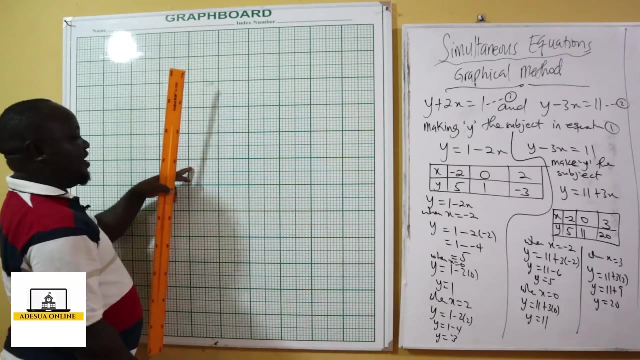 from negative 2 to positive 2, or negative 2 to positive 3.. So assuming I have, let's say, negative 4 here, Negative 3, negative 2, negative 1,, 0, 1,, 2,, 3,, 4,, 5, 6.. I can get my x values Now when. 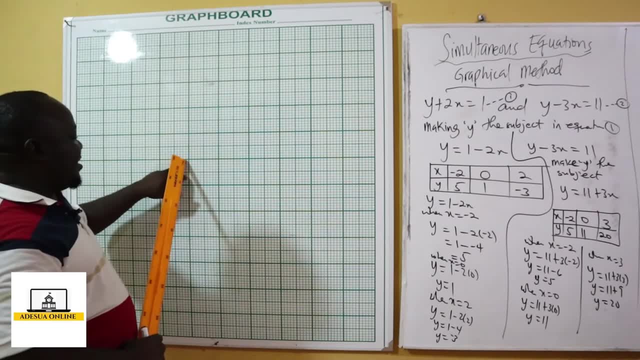 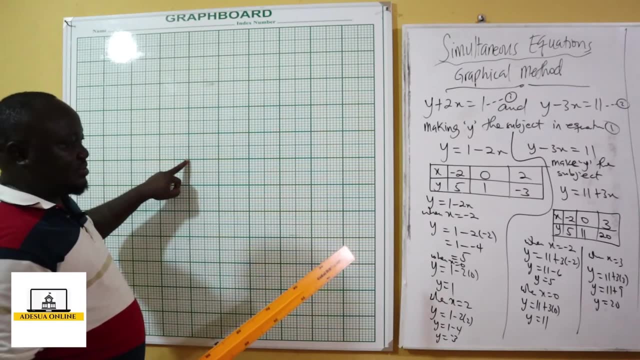 we go to the y values. okay, so I'm dotting this point as my origin for the mean time. Then I go for my y values. The highest value of y is 20.. Okay, So if 2 centimeters to 2, 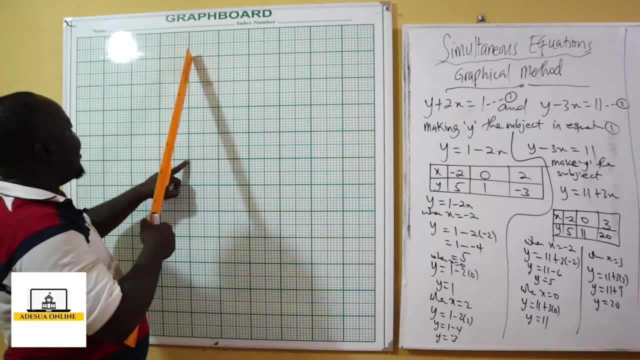 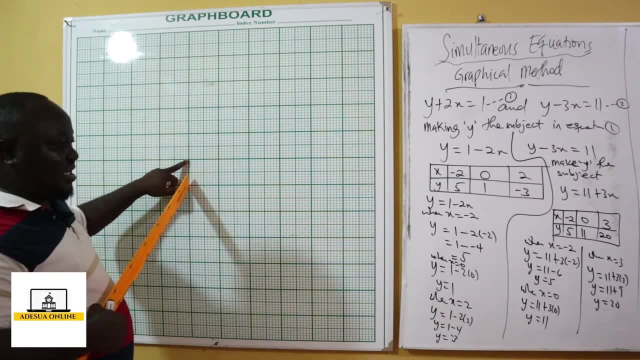 units, then I can have 22,, 20,, 18,, 16,, 14. 12.. Do we have any negative values? Okay, no, So 12,, 10,, 8,, 6,, 4,, 2,, 0. So I can have. 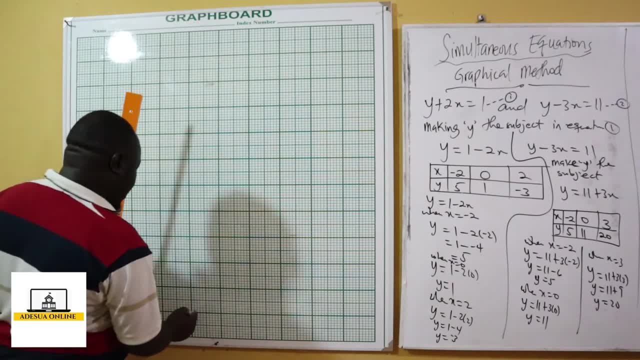 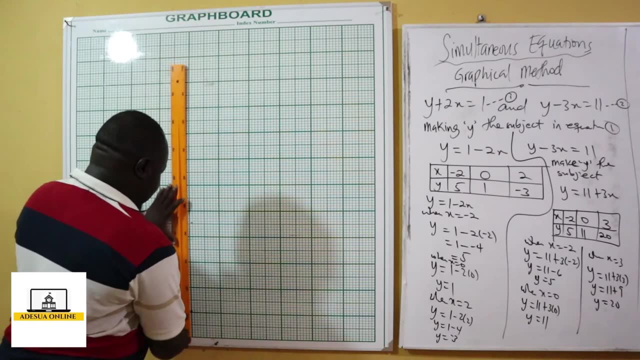 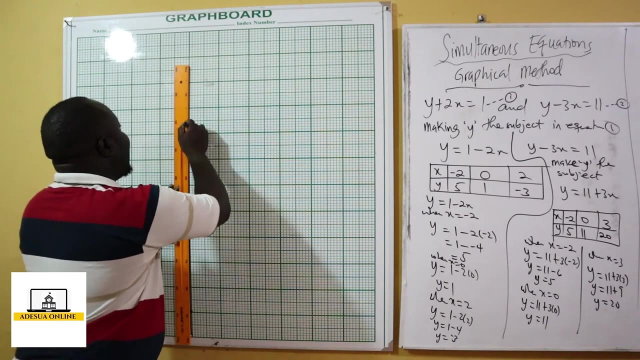 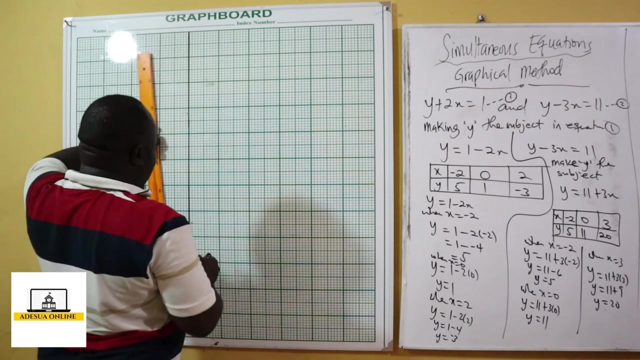 my origin here, So I'll have this point as my origin. So now I'm going to draw my straight lines. That's my x and my y-axis. So I have my y-axis here, Then I level it, So I have this as my y-axis. So if this is my y-axis, I have this as my y-axis. Then 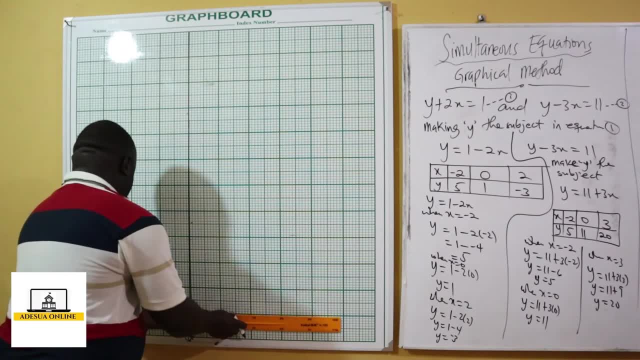 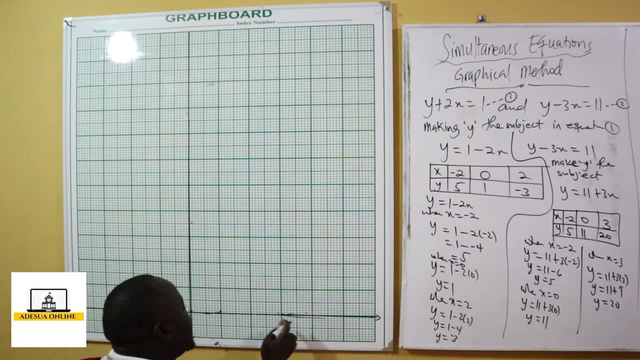 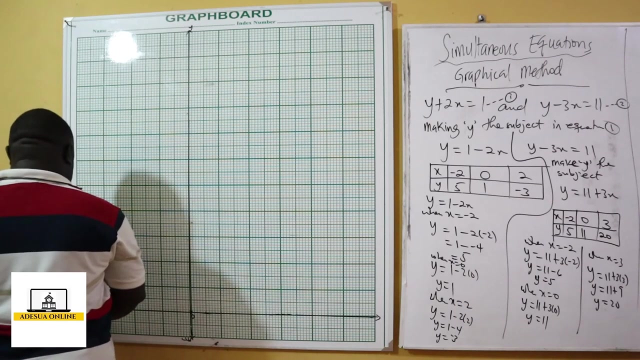 my x-axis will be here. I have my x-axis here. So this is my x-axis. This is my origin 0.. This is my y-axis. I have my negative y here, my negative x, and then this is my positive x. So we are told 2 centimeters to 1 unit on the x-axis. So I 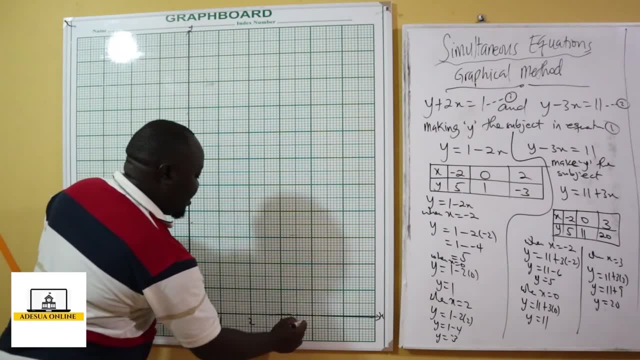 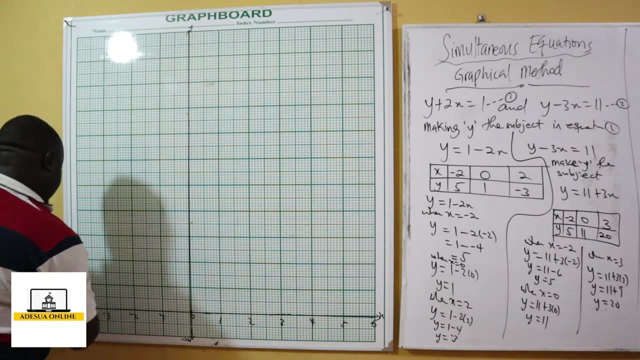 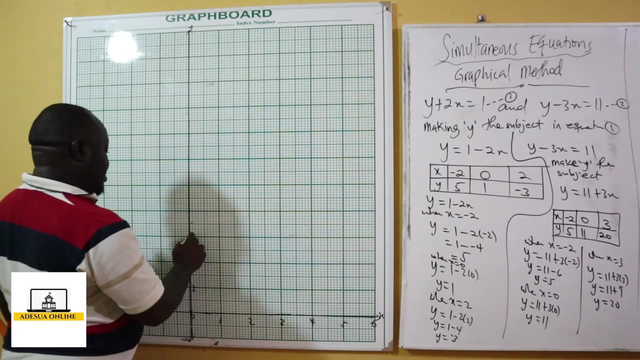 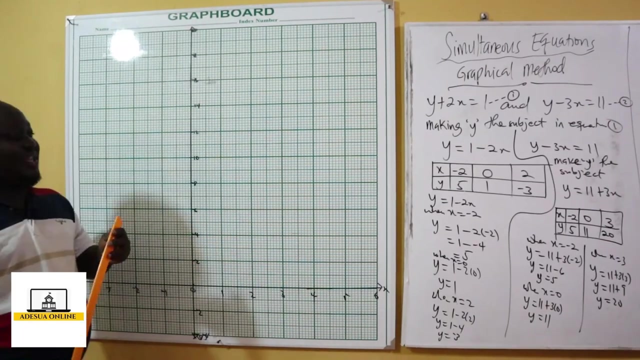 have 1,, 2,, 3,, 4,, 5, 6.. Negative 1, negative 2, negative 3, negative 4.. Then 2 centimeters to 2 units on the y-axis: 2, 4,, 6,, 8,, 10,, 12,, 14,, 16,, 18,, 20.. With the given values, x is negative 2 and y is 5,. 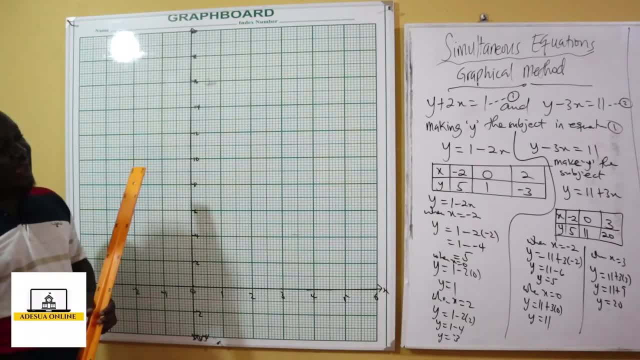 x is 0,, y is 1, and x is 2,, y is negative 3.. We are going to plot this point on the Oxy plane. So when x is negative, 2, y is 5.. So we have negative 2, 5.. So negative 2, 5, we have it. 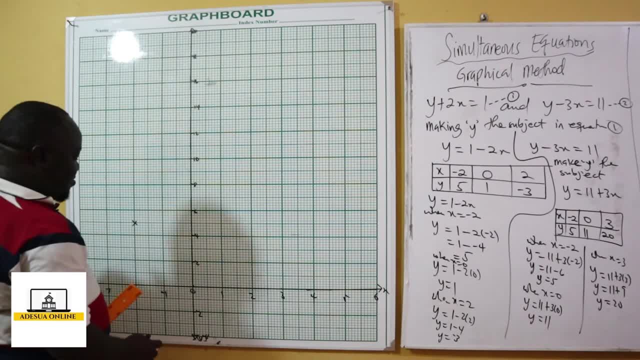 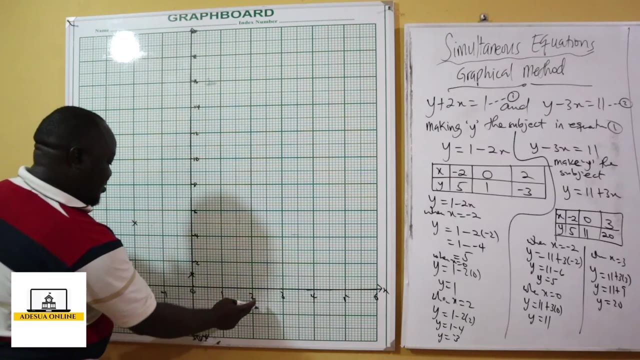 here, in between 4 and 6.. Then we have 0,- 1. When x is 0,, y is 1.. This is 0, 2. So in between 0 and 2 is 1.. So 0, 1.. And then, when x is 2, y is negative. 3. When x is 2, y is negative. 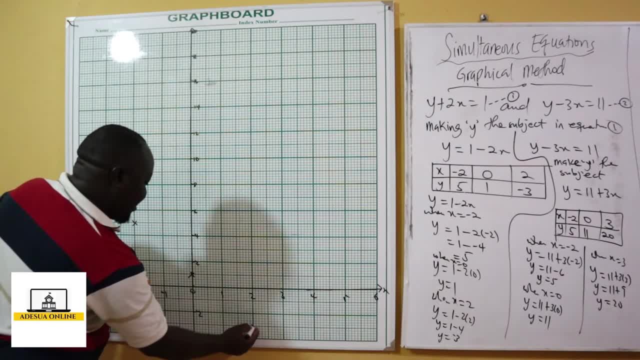 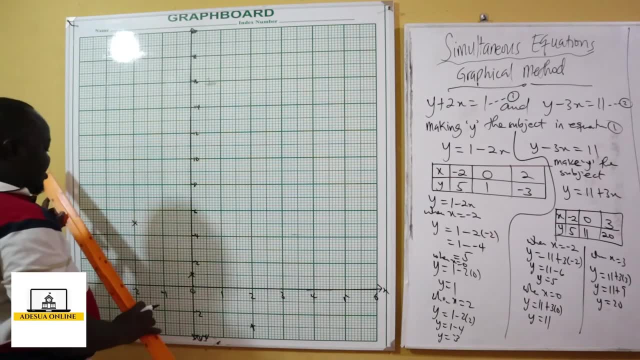 3. This is negative 2, negative 4. We have negative 3 in the middle. So with these three points we are going to pick our rule and then we rule the straight line. We get the straight line from it, So we make. 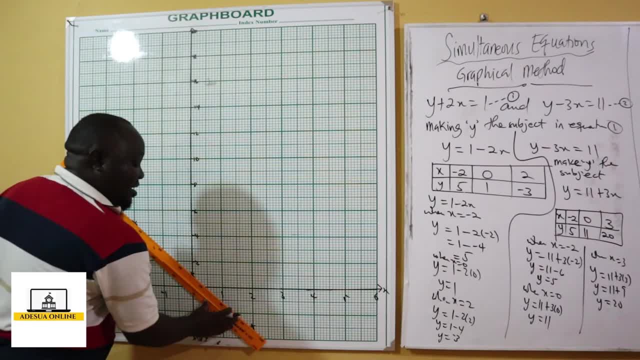 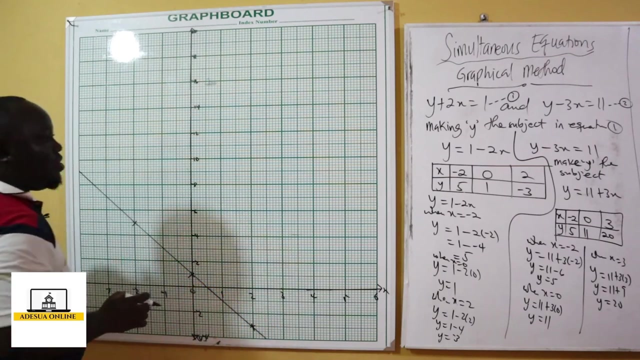 sure our rule is on those three points And I'm very sure the straight line will pass through all the three points. Okay, So we are going to rule the straight line from one end to the other. So we have 2.. So we have this as our straight line. So we have our straight line, for y is equal to 1. 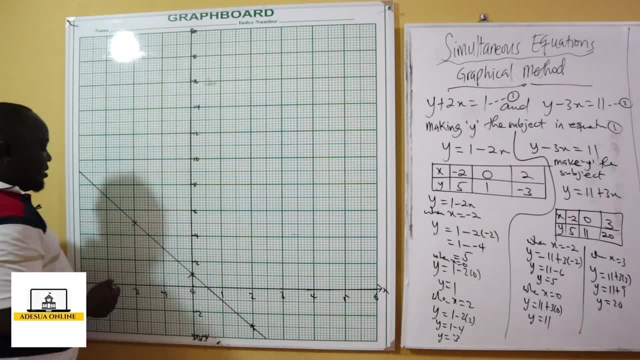 minus 2x or y plus 2x is equal to 1.. So this is the straight line, for y plus 2x is equal to 1.. Then we move to the second point, or the second equation: y minus 3x is equal to. 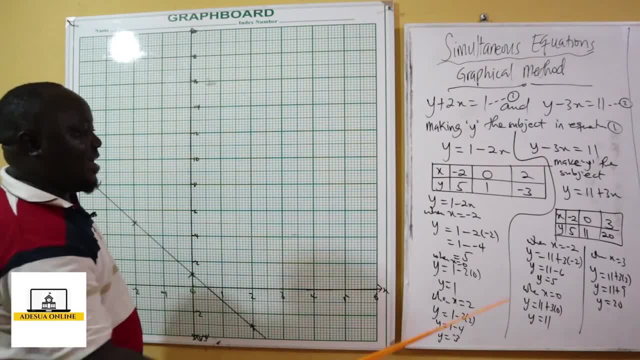 11.. So we are saying when x is negative, 2, y is 5.. When x is 0, y is 11.. And when x is 3, y is 20.. So we have negative 2, 5. x is negative, 2, y is 5., Which is the same point. 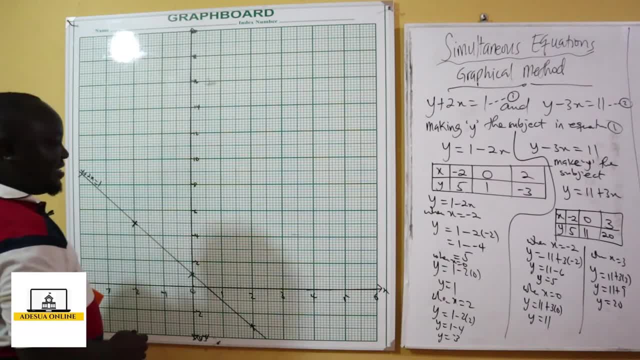 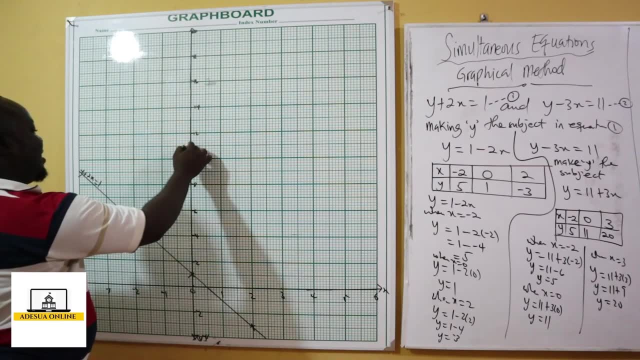 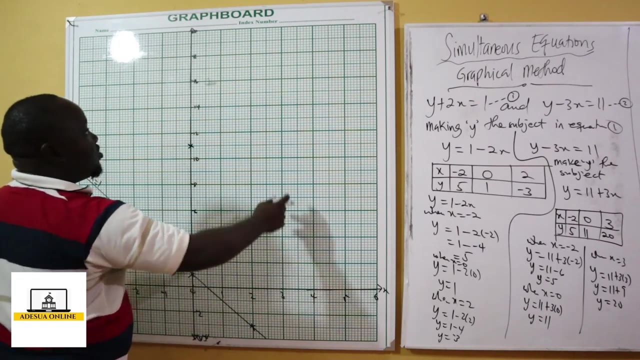 as this: Negative 2, 5.. Then we have x is 0,, y is 11.. 0, 11.. So we have 0, 11 somewhere here It is between 10 and 12.. And then when x is 3,, y is 20.. So 3, 20 is up here, 3,. 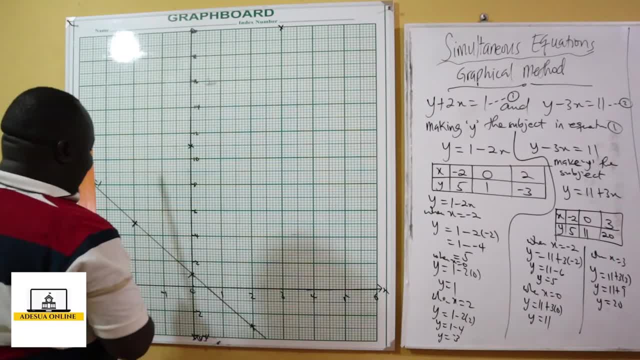 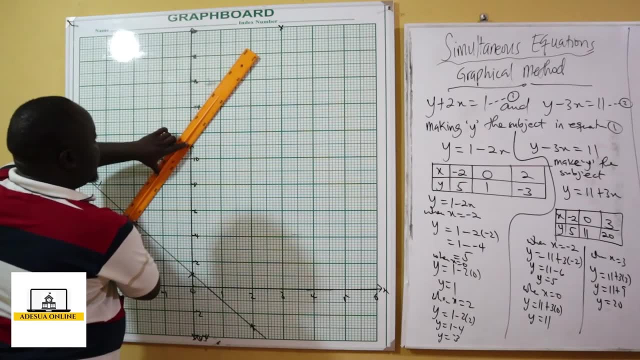 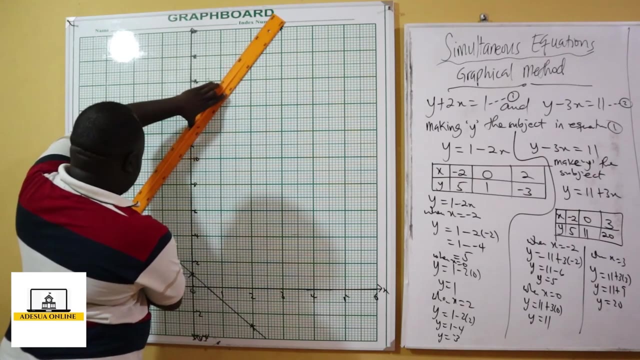 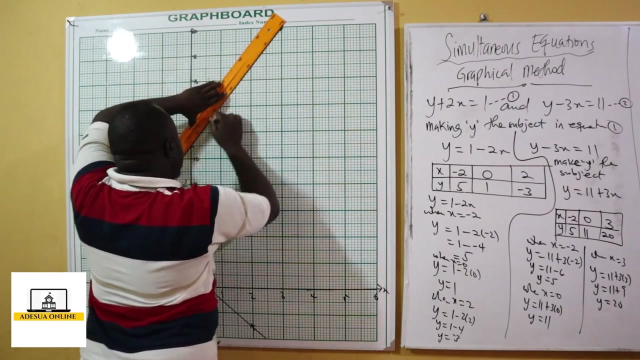 20.. And we are going to pick our rule and then we draw the straight line. You remember, it starts from this point. It starts from this point, So we shall have this, So we shall have our straight line, straight line as this: So this is the straight line of